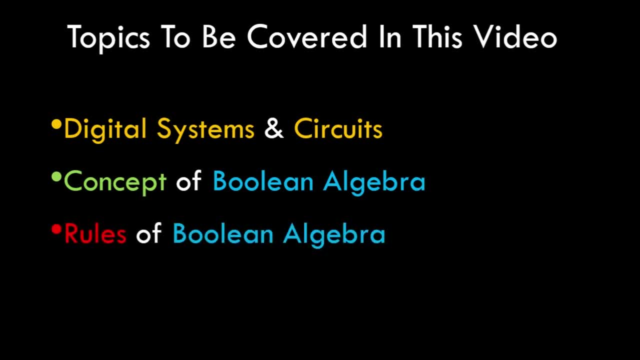 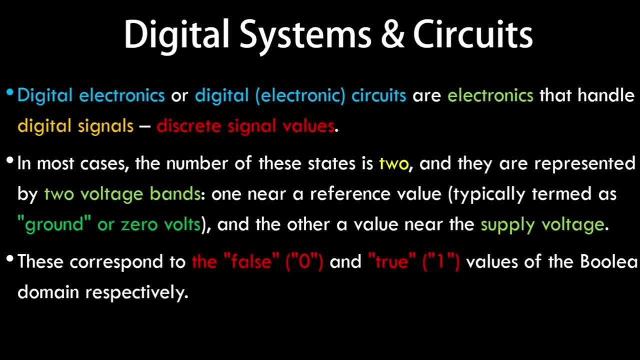 learn some of its rules. So let's understand what a digital circuit is. a digital system or a circuit means. Digital systems or circuits are systems that function with digital signals. Now, digital signals are discrete signals, typically having only two states, that is, high state and low state, usually denoted by the binary number 1 and 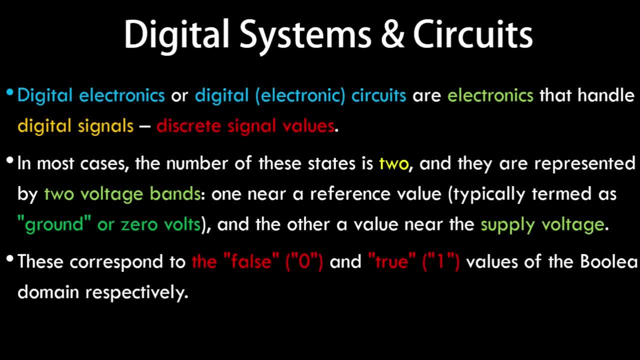 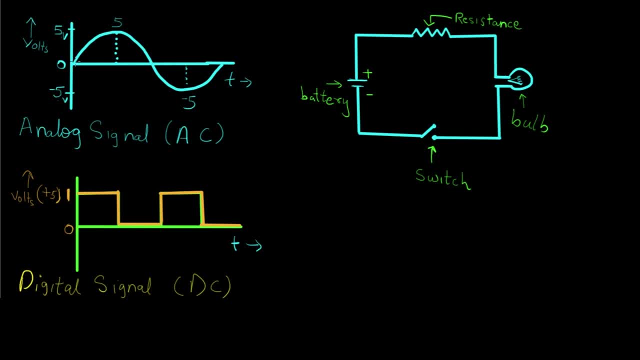 0 respectively. So let me quickly show you an example of digital circuit. Okay, so, as you can see, the first one first diagram is an analog signal, which means that this curve that I have just drawn is an alternating current which variates from minus 5 to plus 5 volts. 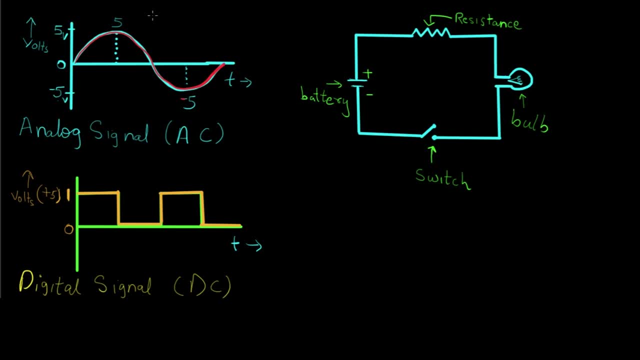 Now this is termed as an analog signal. Now, the devices that operate on digital signals, such as your smartphones, laptops, have this waveform. This is called a digital signal. Now, a digital signal has only two values, that is, 0 and 1, which usually corresponds to the 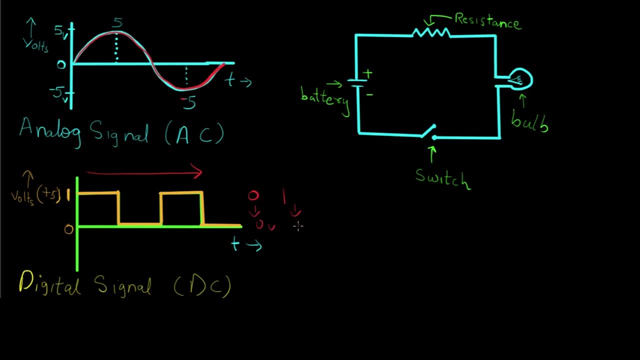 0 volts and 1 corresponds to the higher volts, say, for example, in this case, 5 volts. So all the digital devices, such as your smartphones, laptops, computers, computers, computers, computers, etc. are all digital signals. Now this is called a digital signal, Now a digital. signal has only two values, that is, 0 and 1, which corresponds to the higher volts, So this is called a digital signal. Now, the devices that operate on digital signals, such as your smartphones, laptops, computers, laptops and other devices, usually operate on these digital 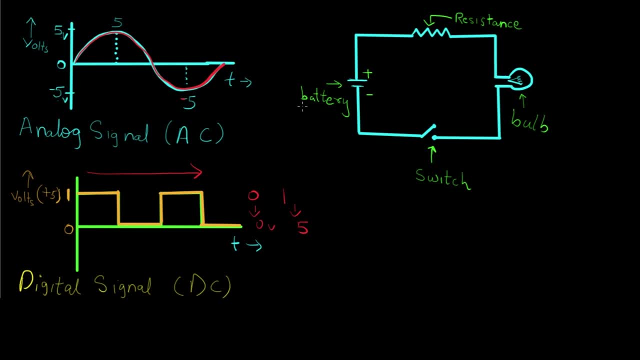 signals. Now I have drawn a basic example of a digital circuit. We have a battery, we have a switch, we have a bulb over here and there is some resistance to that circuit. Now, when this switch is closed, electricity flows from positive to negative and this bulb- 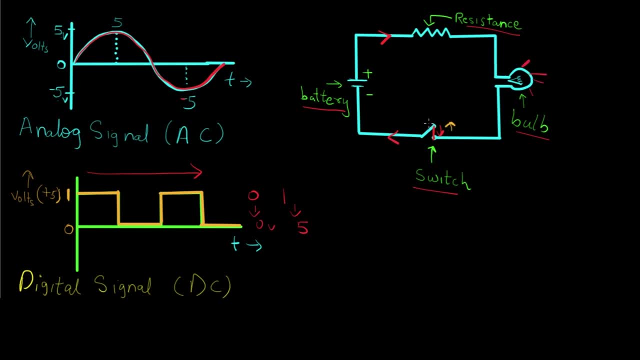 starts glowing. As soon as I off the switch again or break the connection, electricity stops flowing and the bulb stops glowing. So in this case we are applying a digital signal, which is plus 5 volts in this case, for example, and we are switching it on and 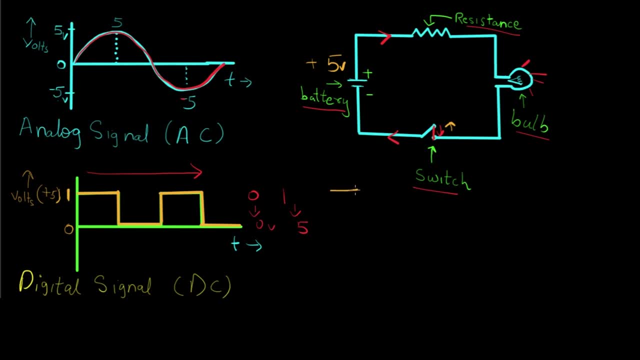 off. So we are switching from plus 5 volts to 0 volts, again back to plus 5 volts to 0 volts. So this is the reason why I drew this waveform. So now that you understand what a digital circuit is and what are digital signals, let's move on to understanding the 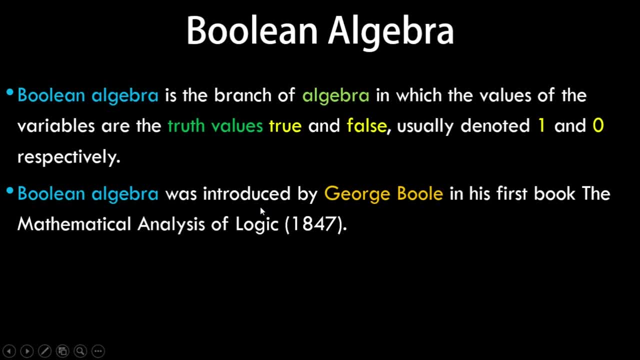 concept of Boolean algebra. Boolean algebra is a branch of algebra in which the values of the variables are truth values, true and false, usually denoted by 1 and 0. It was first introduced by George Boole In 1847,. Boolean algebra is widely used in development of digital electronics and systems.